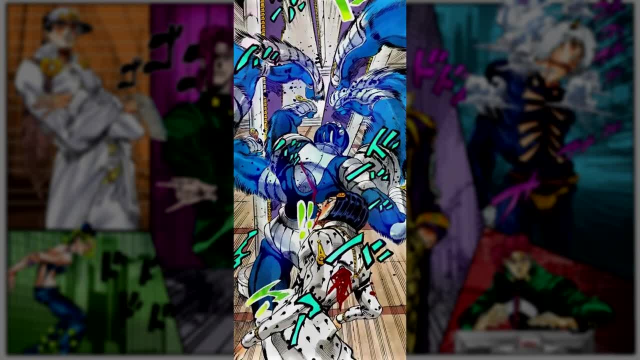 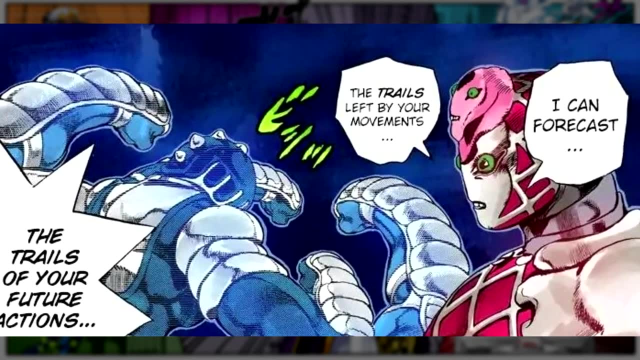 opponent. it would seem as if he is skipping time, but he is not skipping time because no one in the world will experience the same thing as Diavolo. The actions that take place when he activates his ability will experience that period of time. nor would they have any memories of it If Diavolo 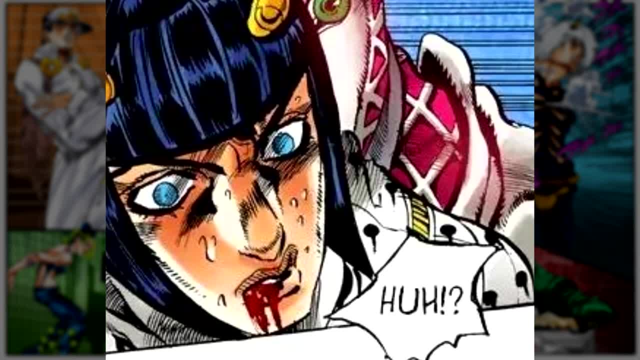 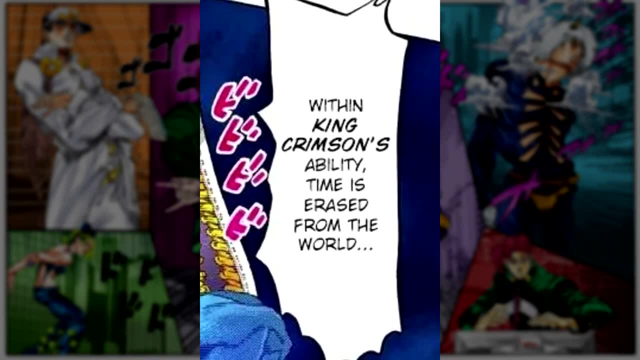 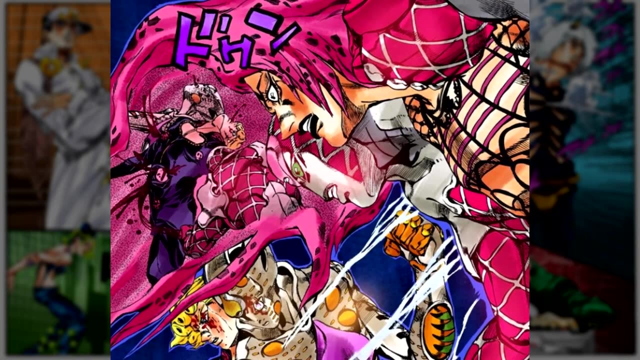 was skipping time as an ability, then everyone would be aware that he is skipping time. The reason why no one has memories of the time is because that time was erased. When Diavolo uses epitaph, he looks 10 seconds into the future, and what he sees cannot be changed. It is guaranteed. 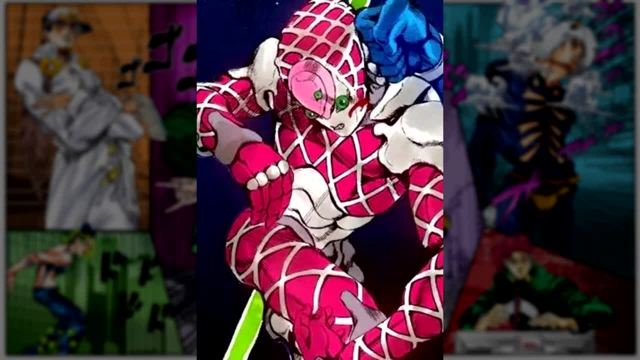 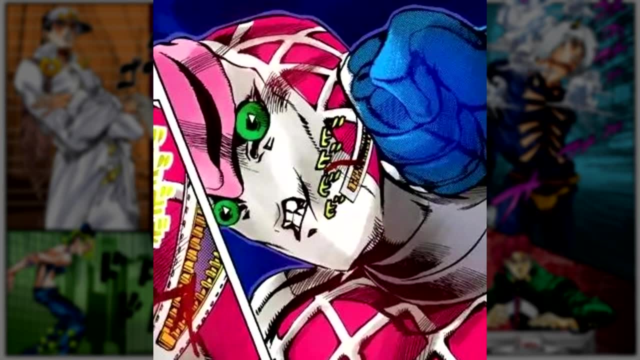 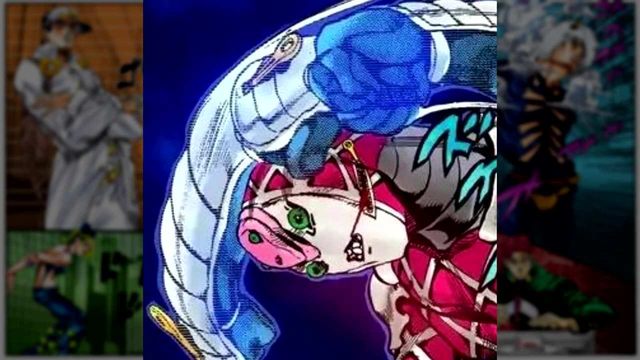 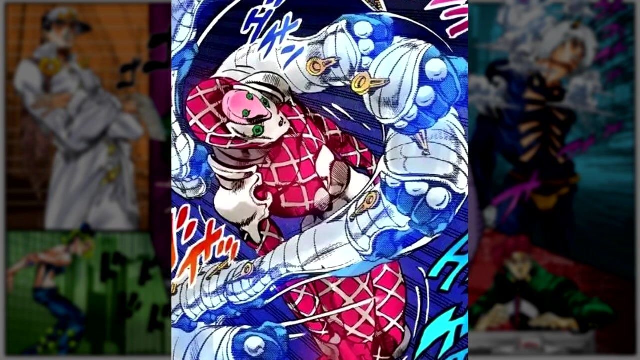 to happen. When King Crimson is activated, it deletes up to 10 seconds of time and whatever happens to him during those 10 seconds is ignored, Meaning that if Naruto were to speed blitz Diavolo and punch him in a nanosecond, it would not matter, because Diavolo would delete or erase the time in which 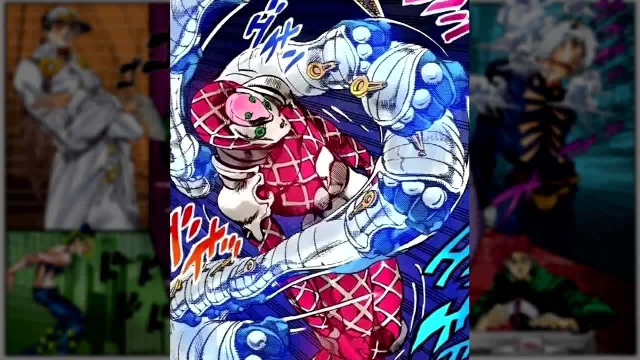 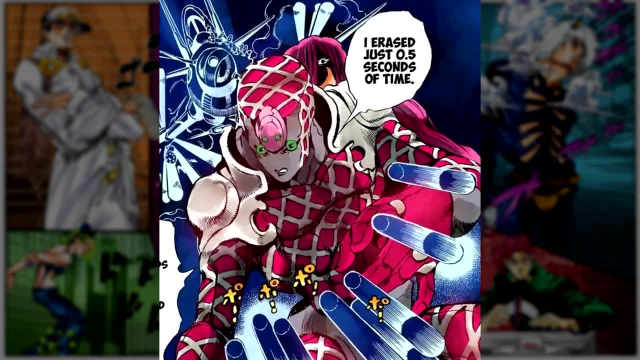 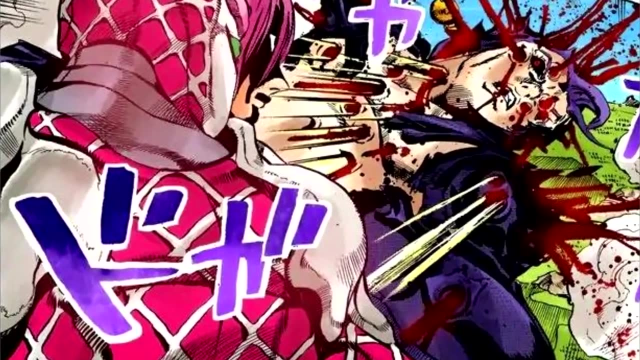 Naruto attacked him, no matter how fast an attack was. So if Diavolo were to speed, blitz Diavolo, it would not matter, because it would be erased. When Diavolo erases time, whatever happens to him is ignored, but anything else that happens will affect everyone else. For instance, when Diavolo 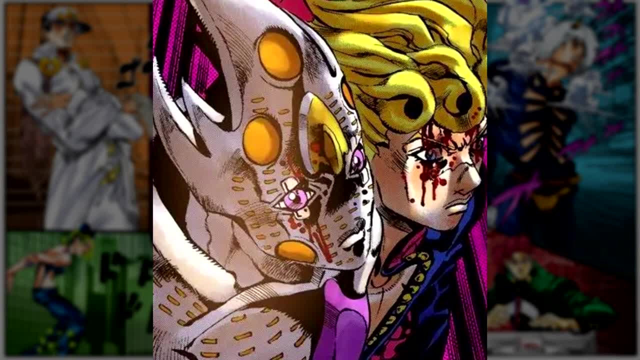 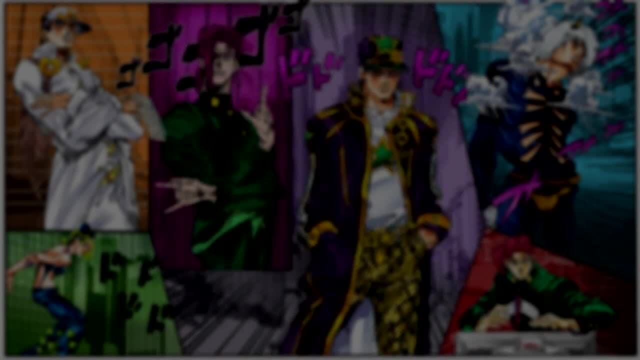 put blood in Giorno's face, it was still able to affect Giorno because it was something that was happening to Giorno and not Diavolo. In a fight, Diavolo is invincible. This is why his most suitable death was a Death Loop, because, while in a death loop, if Diavolo were, 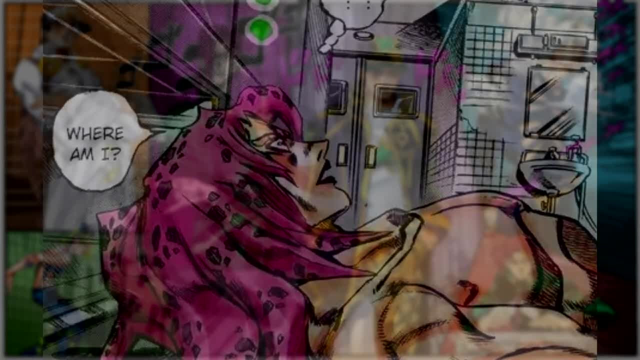 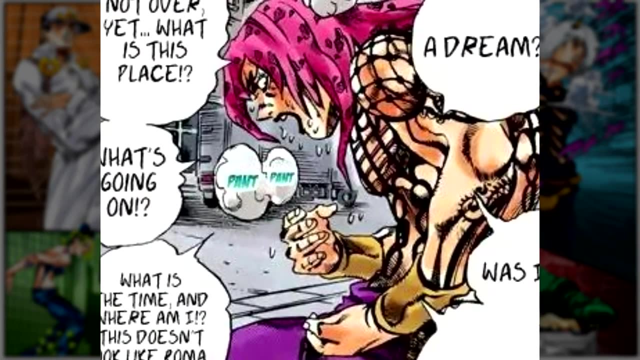 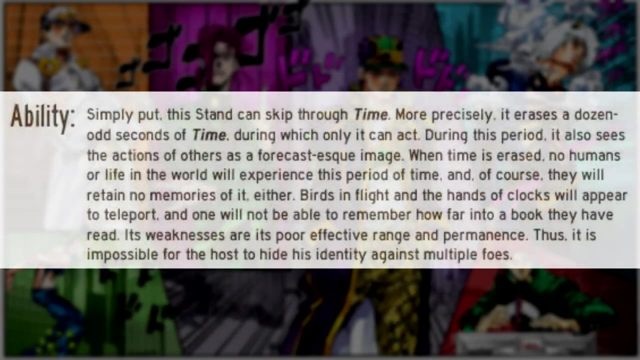 to erase the time in which he died. he would not die, But by being in a Death Loop he would just go back to the loop and die again and again. The Death Loop makes King Crimson's ability meaningless. King Crimson can skip through time. More precisely, it erases a definite way in the 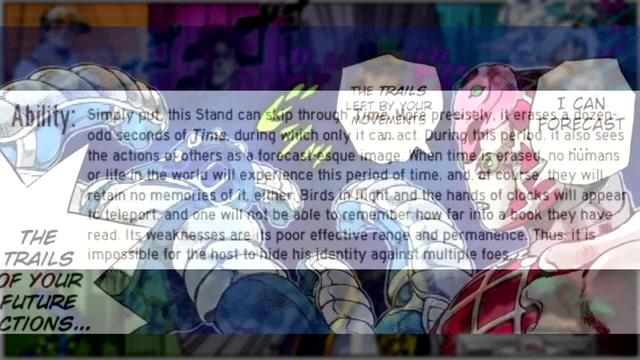 world and then he goes againstЕё. But if you do take into account that T4 change is ins physico's picture in the use of r1, then changes these. 원단줄quorm can't spinning an" dozen odd seconds of time, during which only it can act during this time period. 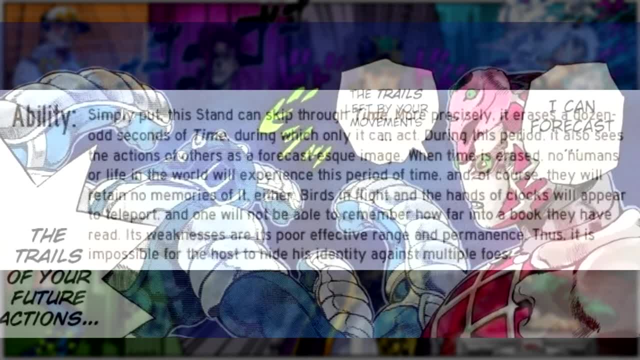 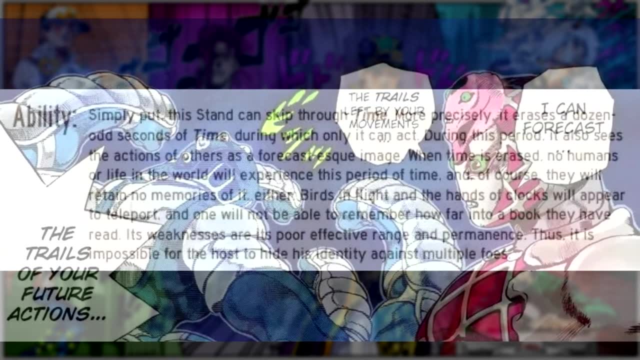 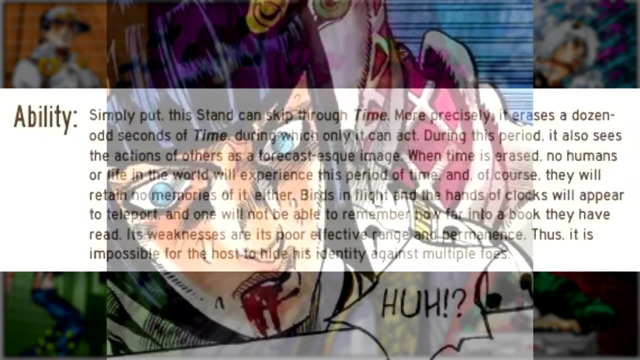 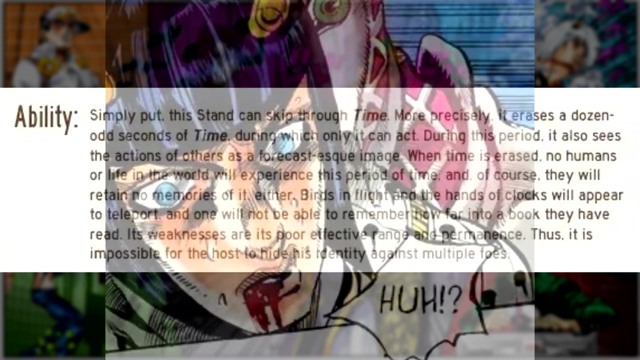 It also sees the actions of others as a forecast-esque image When time is erased. no humans or life in the world will experience this period of time and, of course, they will retain no memories of it either. Words in flight and the hands of a clock will appear to teleport and no one will ever remember. 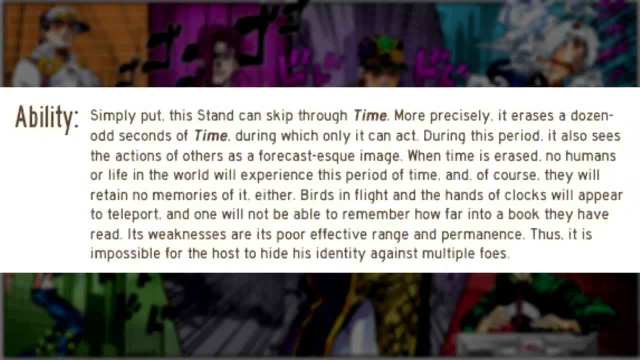 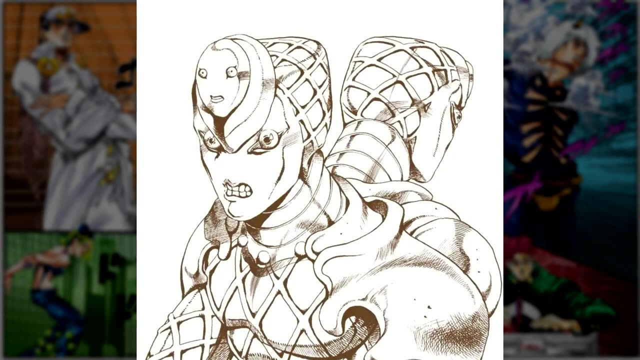 how far into a book they have read. Its weaknesses are its poor effective range and permanence. thus it is impossible for the host to hide his identity against multiple foes. If King Crimson was skipping time, he would be able to move forward or backward through. 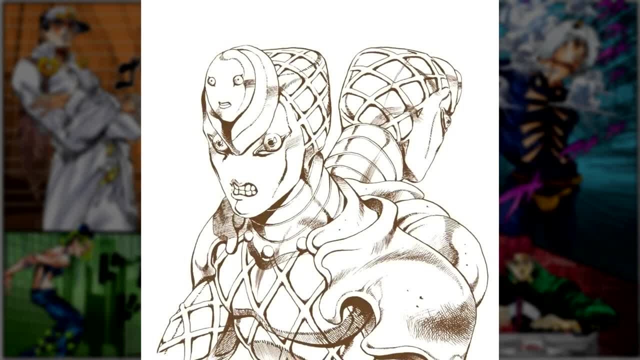 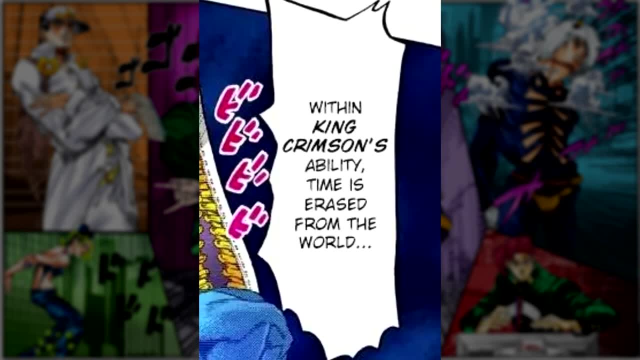 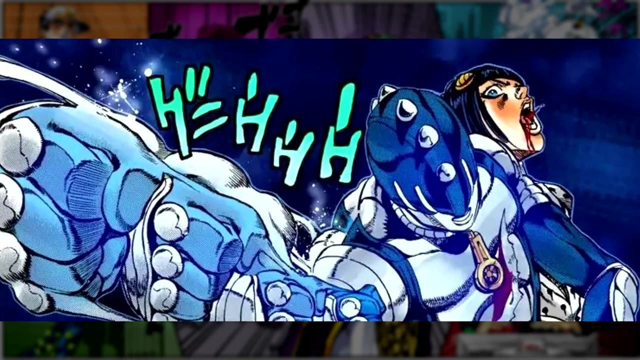 that time frame. But, as I mentioned before, Diavolo does not skip time. Diavolo erases time, but that erasure in time causes time to skip to the point in which the event Diavolo wants to erase is erased. 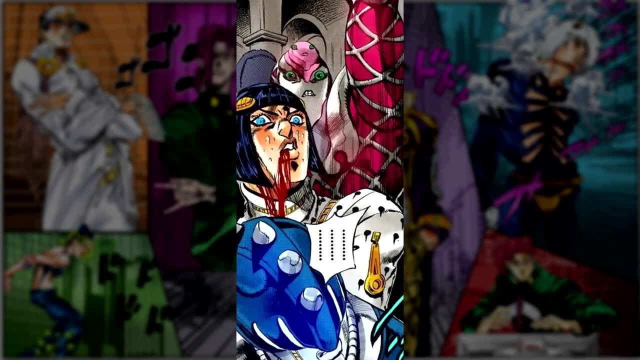 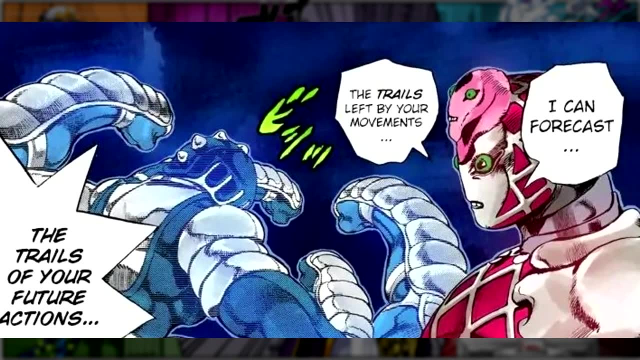 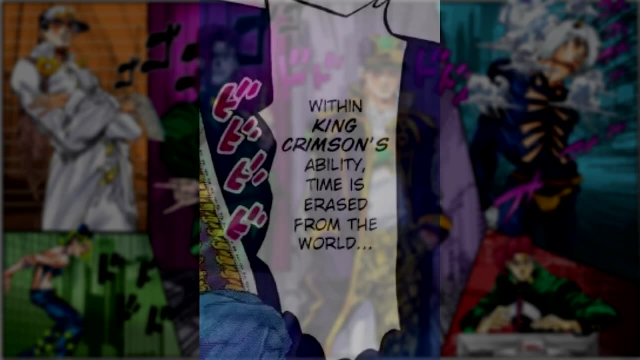 And people keep confusing that as to if the skip created through Diavolo erasing time is his ability to skip time, Which his ability is not. His ability is to fucking erase time. Look, I eradicated time and forced it to skip. 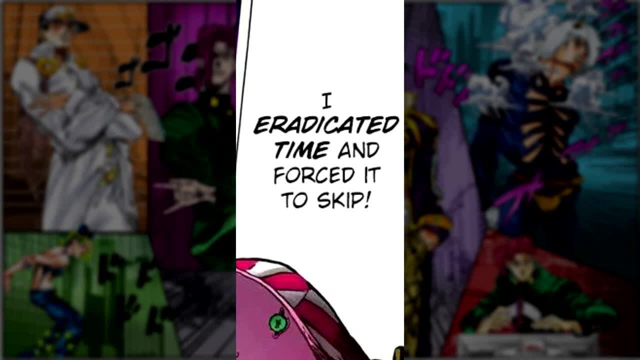 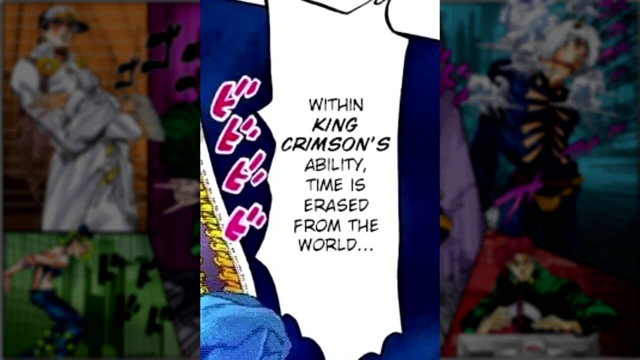 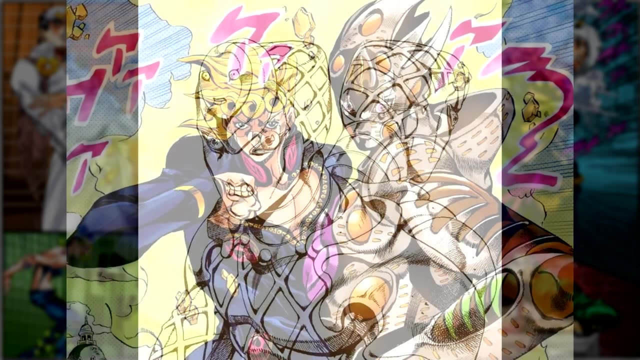 Diavolo, erasing time would cause time to skip. Diavolo is not skipping time. Diavolo's ability is to erase time. Diavolo has a broken ability. His ability is so broken that Giorno's Gold Experience Requiem is broken. 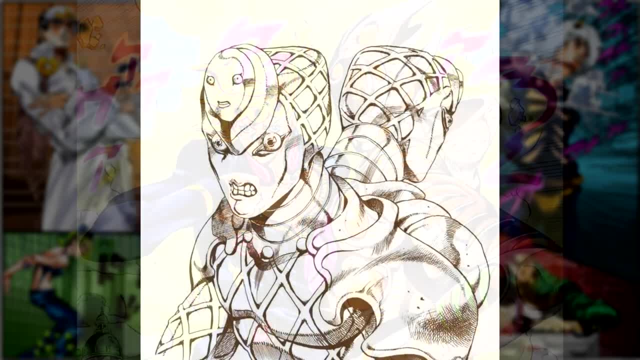 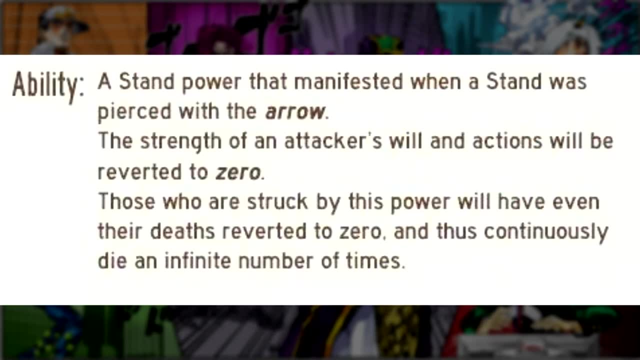 Giorno's Gold Experience Requiem is broken. Giorno's Gold Experience Requiem is broken. Giorno's Gold Experience Requiem is made to be a direct counter to Diavolo's ability. Giorno's ability makes the will and actions of the person he is fighting revert to zero. 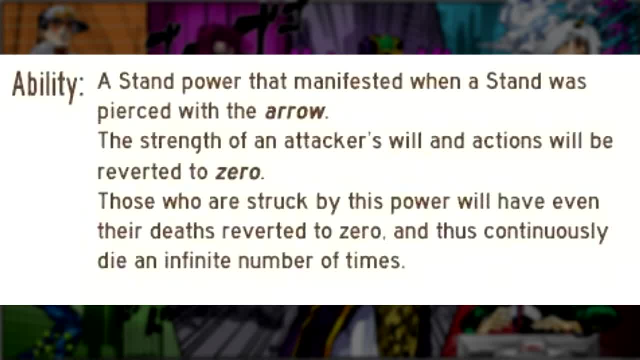 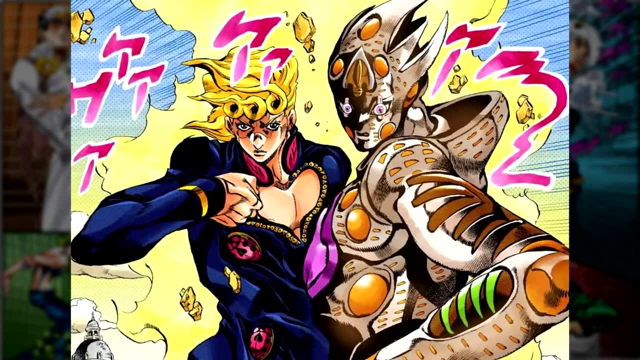 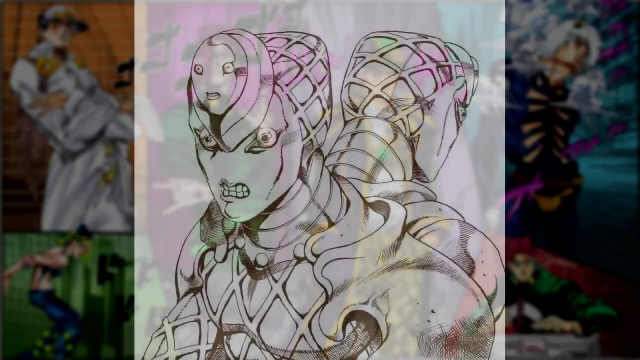 Meaning that Giorno makes whatever you do meaningless. You are essentially nothing. when Giorno uses his requiem, Giorno's ability is the only thing that can stop King Crimson's ability, Because King Crimson is fucking broken. To describe Diavolo's ability in the simplest way possible, let's say: you shoot me with.